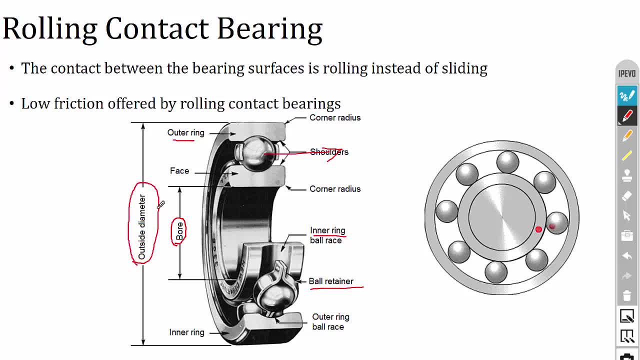 And the maximum outside diameter. This is the diameter of the bearing. So the shaft will be inserted on the bore and the shaft will rotate along with the inner race and the outer race is placed with your stationary part and in between the outer race and inner race the balls will be there and the balls will rotate so that the friction 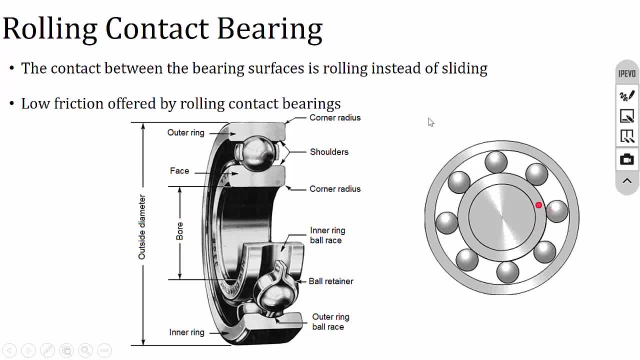 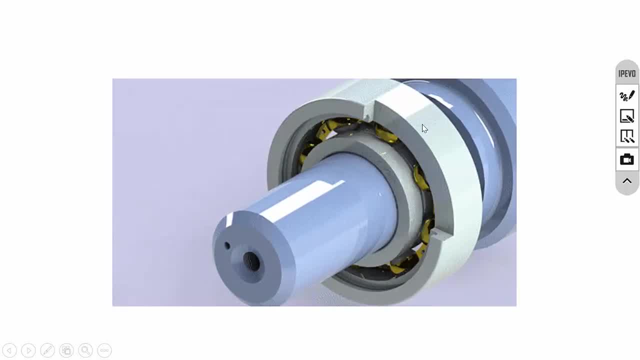 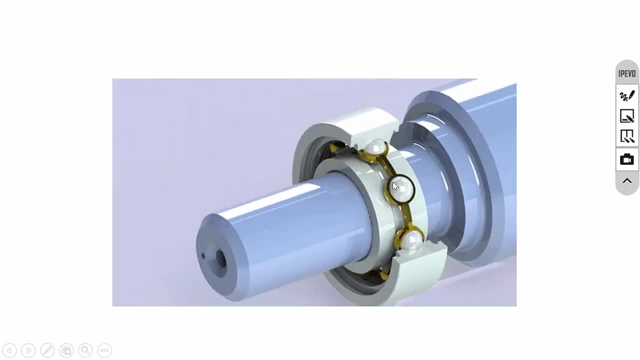 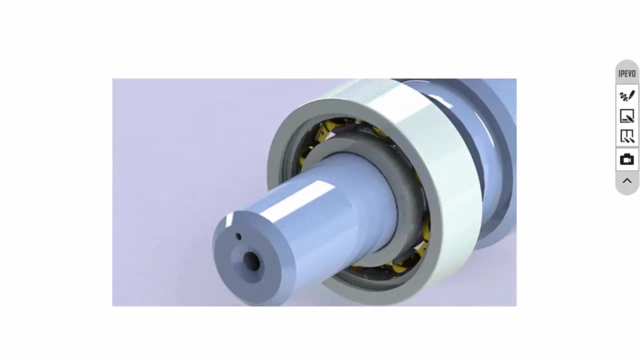 will be reduced. So you can see an animation of rolling contact bearings. So this is the inner race And this is the outer race. So here you can see the balls and the retainer is used to keep the ball in position. So in case of sliding contact bearing, there will be no rollers or balls and only lubrication. 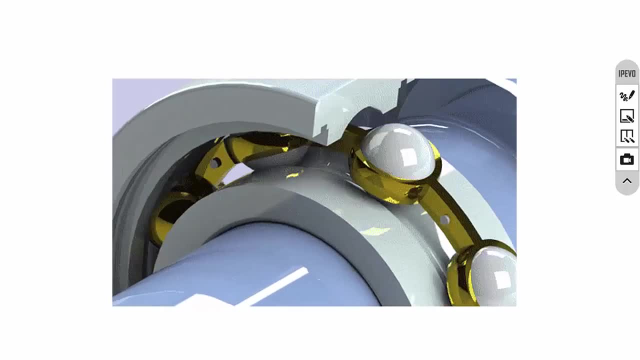 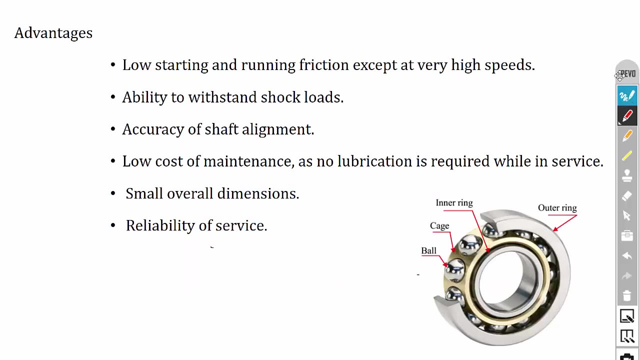 is used to separate the journal from the outer bearing. So here balls and rollers are used. So the advantages of rolling contact bearing: First one: Low starting and running friction, except at very high speed. because of using the balls in between inner race and outer race the friction will be very low, except at high speeds. 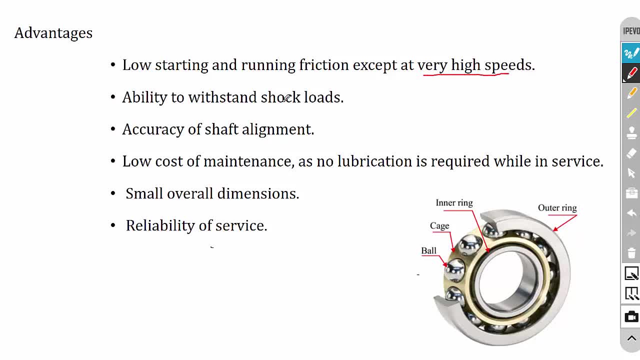 For high speed operations we can go for sliding contact bearings. You can able to withstand high amount of shock loads. Then the accuracy of shaft alignment will be high, because in case of sliding contact bearing At initial stage the journal will be at the bottom point. 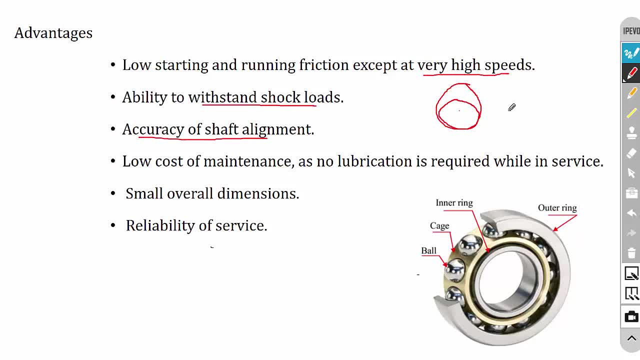 So the center of gravity will not match with the bearing center of gravity. But when it starts to rotate because of the centrifugal force, the journal will come to its center. in case of sliding contact bearing, So the alignment will be varying. but in case of rolling contact bearing, the inner race. 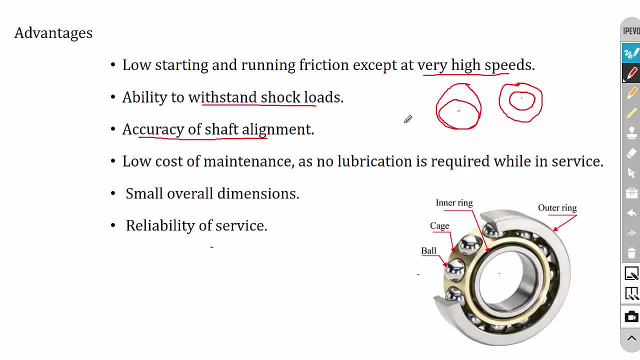 is stationary one and it will not move up and down, so that the shaft alignment will not be varying. Low cost of maintenance, as no lubrication is required, So the maintenance cost is very minimum because we don't need to provide any lubrication. Then small overall dimensions. 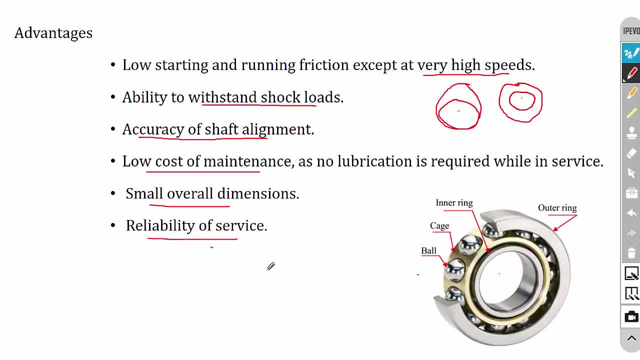 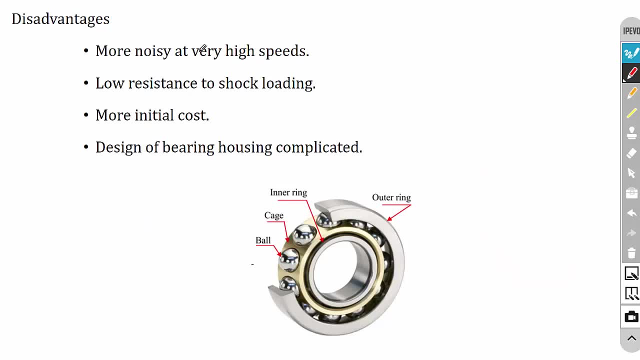 Then reliability of service. So these are all the advantages of using rolling contact bearing. Then these are all the disadvantages. So the first one is more noisy at very high speeds because the ball has to rotate, and when it touches with the outer bearing, So the ball has to rotate. 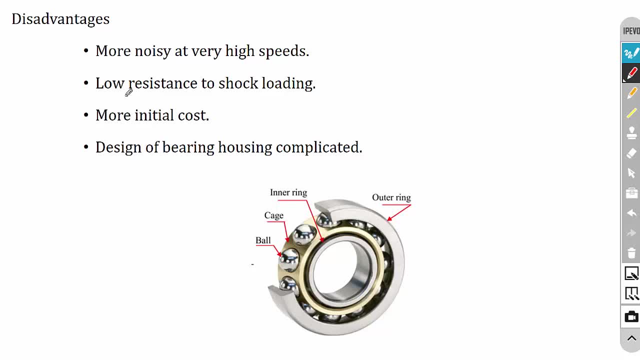 When it touches with the inner and outer rays it will produce some unwanted noises. Then low resistance to shock loading. So if the shock is produced then it will damage the balls. Then more initial cost comparing with the sliding contact bearing. So design of bearing hosing is complicated. 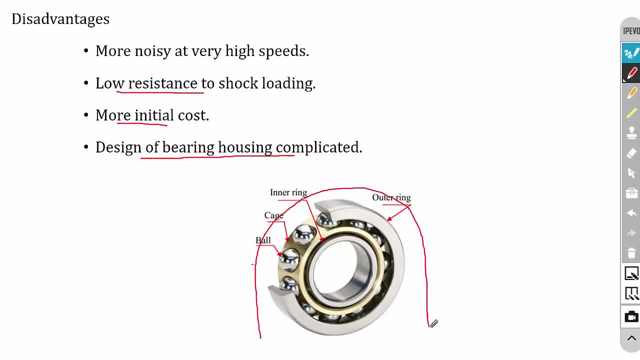 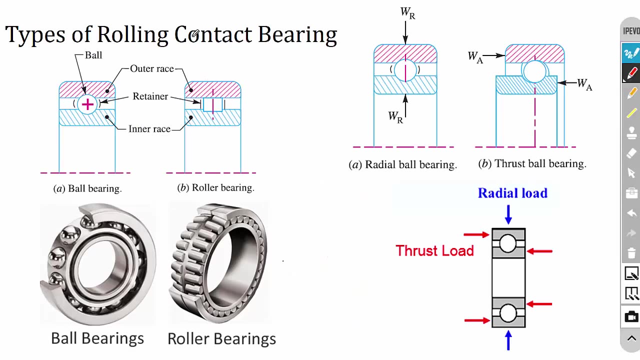 So around the bearing we have to provide a bearing hosing like this to keep the bearing in a stationary part. Ok, So design of bearing hosing is a complicated one in case of rolling contact bearings. So next, the type of rolling contact bearings. 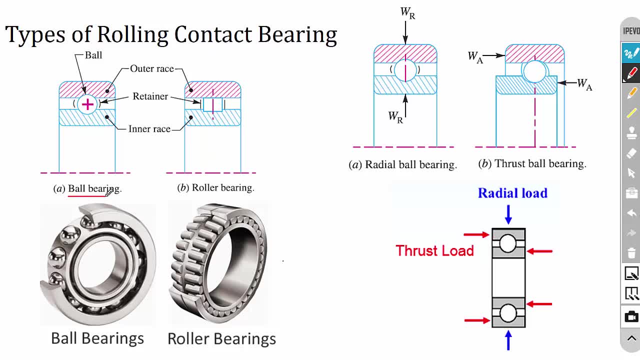 So the rolling contact bearings can be splitted into two. One is ball bearing and another one is roller bearing. In case of ball bearings, the balls are used in between the inner rays and outer rays. In case of roller bearings, instead of spherical ball, a cylindrical roller will be used to. 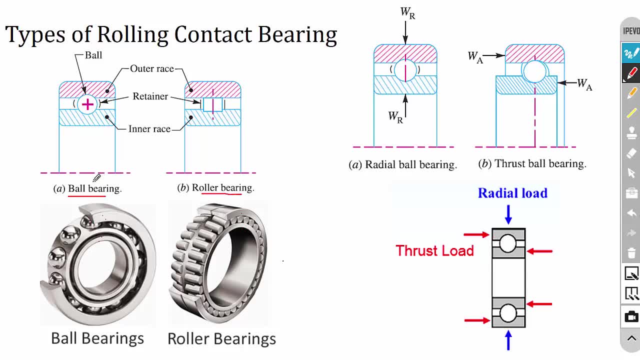 separate the inner rays and outer rays. So that is the difference between ball bearing and roller bearing. So first we will focus on the ball bearing. The ball bearing is further splitted into two. One is radial ball bearing and the other one is thrust ball bearing. 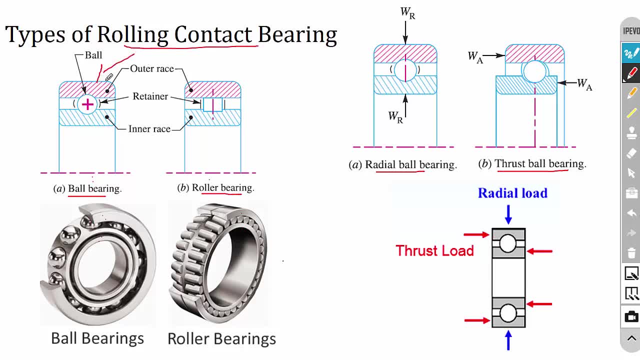 So in general, the rolling contact bearing is splitted into two, that is, ball bearing and roller bearing. Further, this roller bearing is splitted into two. One is radial ball bearing and the other one is thrust ball bearing. Ok, in case of radial ball bearing, the bearing is to is designed to take only the radial loads, so that 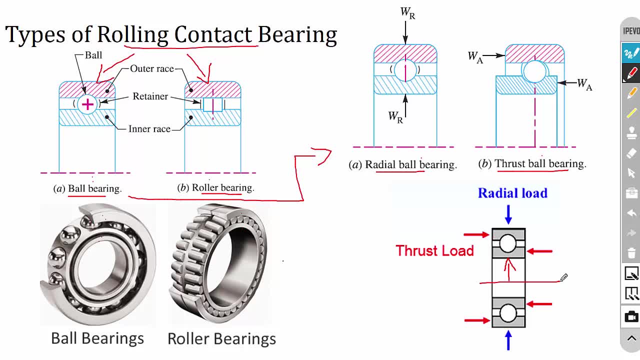 is the loads acting to the perpendicular to the axis of the shaft, so that is radial load. so this radial ball bearing can able to withstand only the radial loads in case of thrust ball bearing. so the ball bearing is designed to take the thrust loads. so thrust load means axial load, the load. 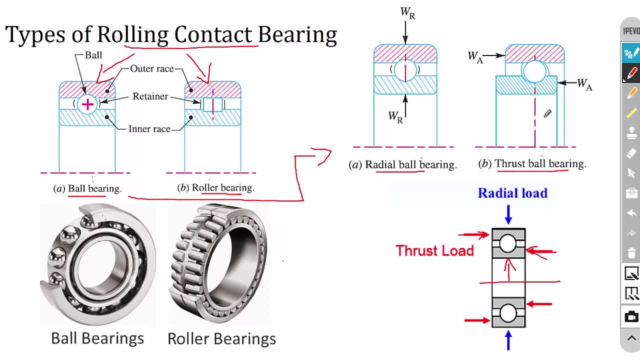 will be acting parallel to the axis of the shaft. okay, also in some some of the thrust ball bearings we can apply both thrust load as well as radial load. okay, so this radial ball bearing and thrust ball bearing have small uh design changes in its constructions, so we'll see that in the next slide. 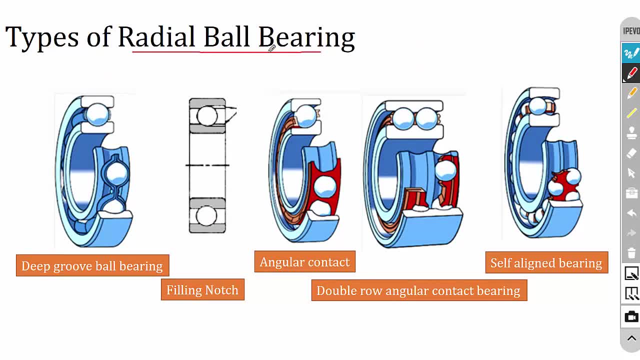 so these are all the types of radial ball bearing. so the radial ball bearings are used to take up only the radial loads. so the first one is deep group ball bearing, so it's the most common one. so the balls are used in between inner race and outer race and a ball retainer is used to keep the balls in position. so that is deep groove. 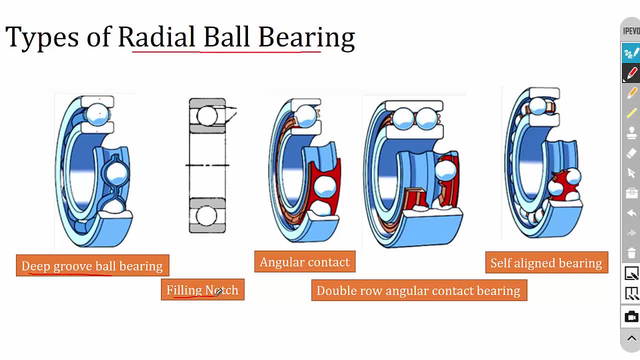 ball bearing. in the case of fillet notch bearing, a small notch is produced on both inner race and outer race to keep the balls in position. you can see the image. a small notch is produced here. so that is fillet notch bearing. then the next one is angular contact bearing. so in case of angular 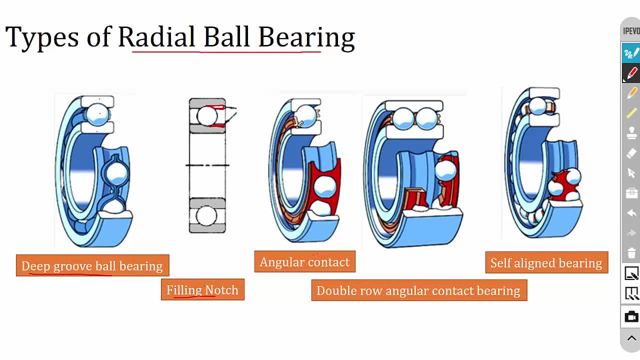 contact. the inner rays and outer rays will be in angular contact with the balls. you can see that. so if you draw the cross section, then it will be like this: so this is the top part and this is the bottom part. so your balls will be like this, so this can able to withstand radial loads as well as. 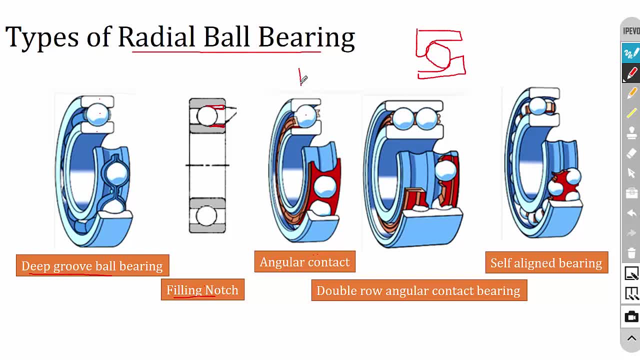 this, so this can able to withstand radial loads as well as some amount of thrust load in only one direction. for example, if you see this image, if you apply a thrust load in this direction, then it can able to withstand the minimum thrust load, but if you apply the thrust load in opposite direction, then 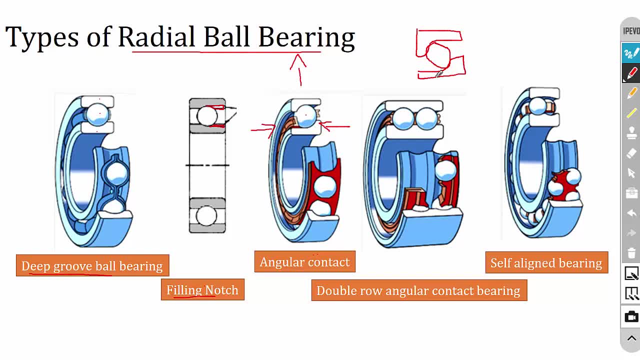 it cannot able to withstand the load because it will go in this direction. so the ball will not be, will not touch the inner race and outer race. ok, so this angular contact bearing is designed in such a way that it can withstand axial loads as well as a minimum amount of thrust load, I mean. 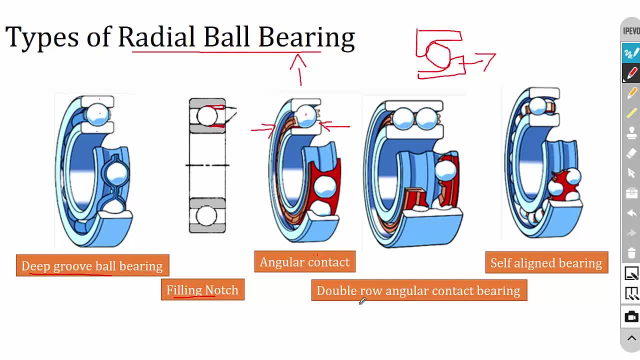 radial load as well as minimum amount of thrust load. so the next one is double row angular contact bearing. so it's, moreover, like your single row angular contact bearing. in single row angular contact bearing, a single row of balls are used. In case of double row angular contact bearing, two rows are used here. 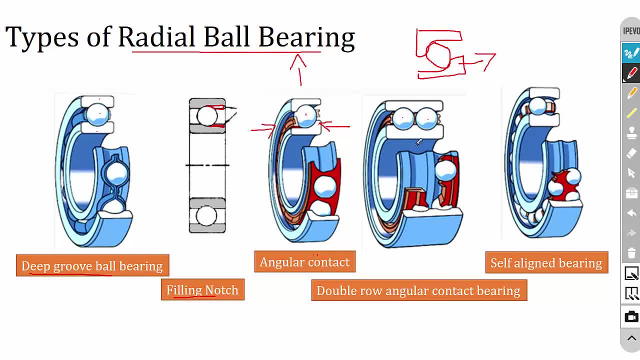 So the load carrying capacity of this double row angular contact bearing is more over twice the load carrying capacity of single row angular contact bearing. Anyway, it will be slightly less than the double times of single row angular contact bearing. Then the next one is self aligned bearing. 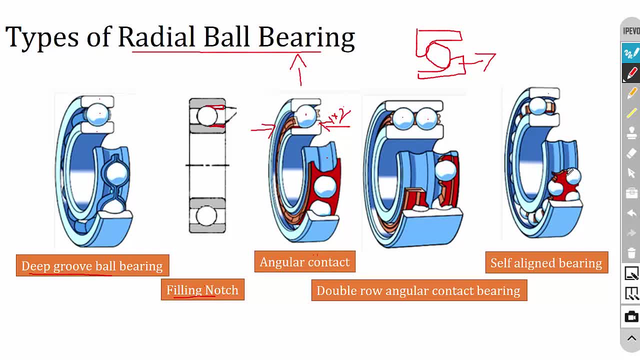 In case of self aligned bearing. so the retainers will keep and retainers and the grooves provided in the inner rays and as well as outer rays will keep the balls in aligned. So it will keep the balls in aligned as by itself. So the standard designation. 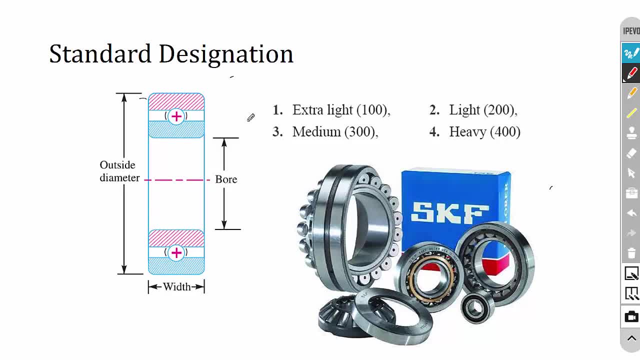 So the bearing standard is very, very important. So the bearings are mostly standardized Based on its load carrying capacity as well as its bore diameter. So if a bearing number starts with 100, then its extra light weight carrying- I mean extra light load carrying bearing. 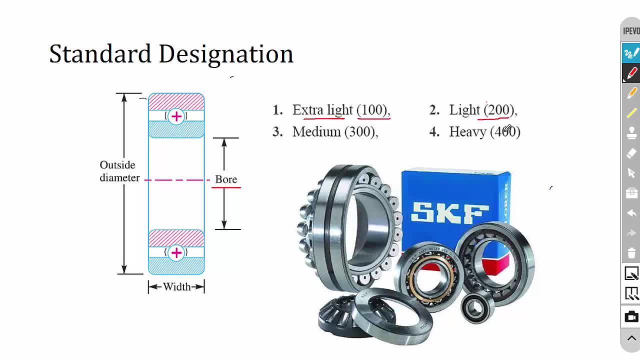 So if it starts with 200, then it can able to withstand light loads. If it starts with 300, then we can apply medium loads. If it is 400, then it is for heavy load applications. Ok, So SKF is a manufacturer of bearing. 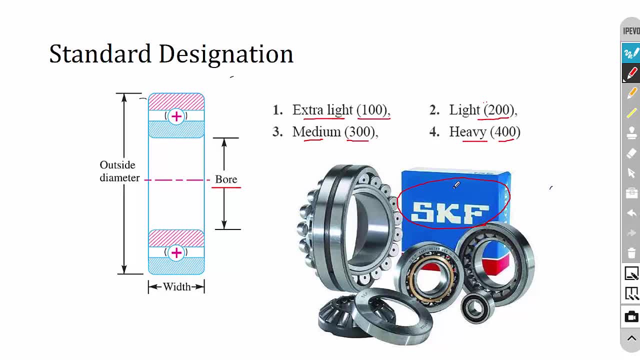 So SKF has developed its own standard and in this design we are going to follow the SKF standards only. and SKF is actually a manufacturer of bearing, So Skwenska Kullankar Fabrikan is the abbreviation for SKF, and this SKF standard is there in. 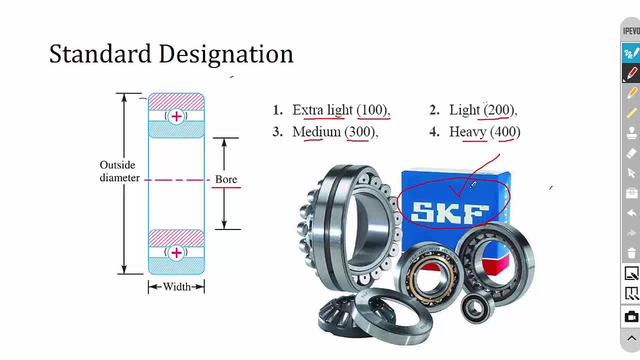 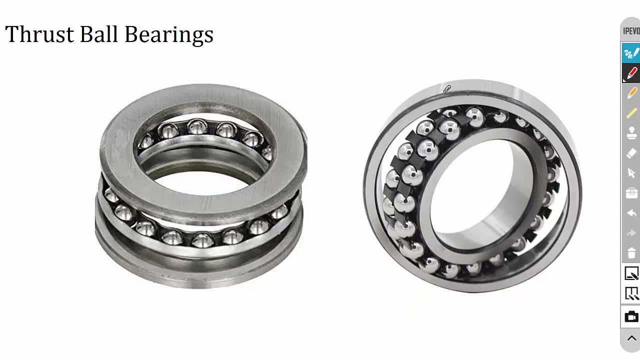 our data book, PSG data book, So we can directly take the standard bearings from our data book. Next one is the thrust bearing. So initially we have seen the radial bearing, So here it is thrust bearing. So in thrust bearings we can apply both axial load as well as thrust loads. 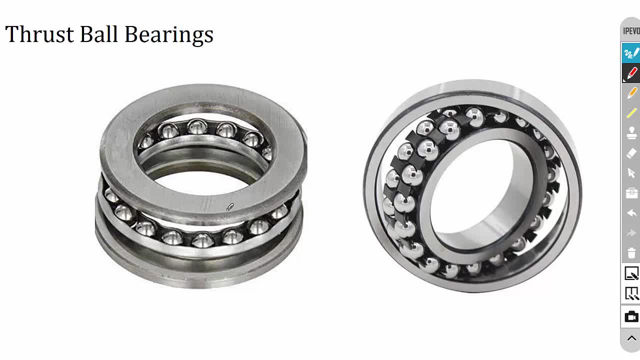 So the design is based on carrying thrust loads as well as the axial load. So this left side image is a single row thrust ball bearing and this image so it has two rows of ball bearings Balls. This is called as double row thrust ball bearing. 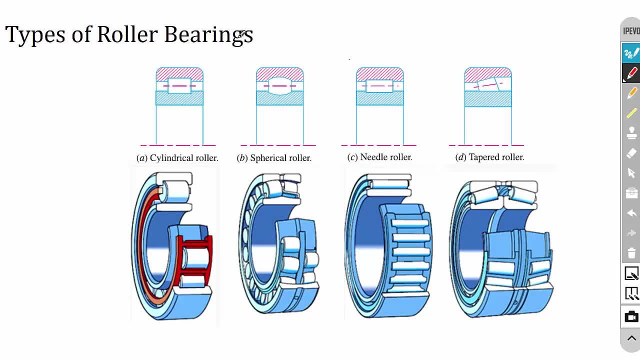 The next one is roller bearing. So in case of ball bearings, so balls are used in between the inner race and outer race. In case of roller bearings, the rollers will be used. So the first one is cylindrical roller bearing, So here a circular cylinder is used in between the inner race and outer race.